by which population is rising and thus is quick industrialization. it is vital to understand how to conduct waste disposal In the realm of today, by which population is rising and thus is quick industrialization. it is vital to understand how to conduct waste disposal In the realm of today. 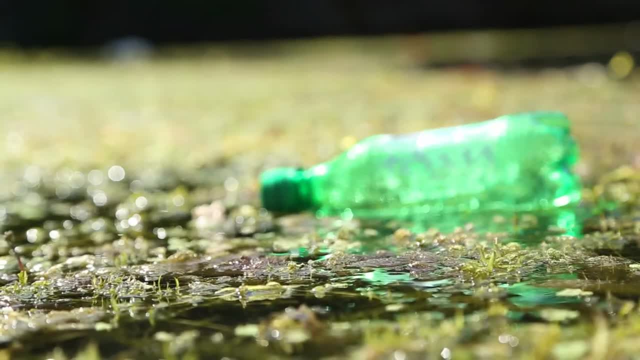 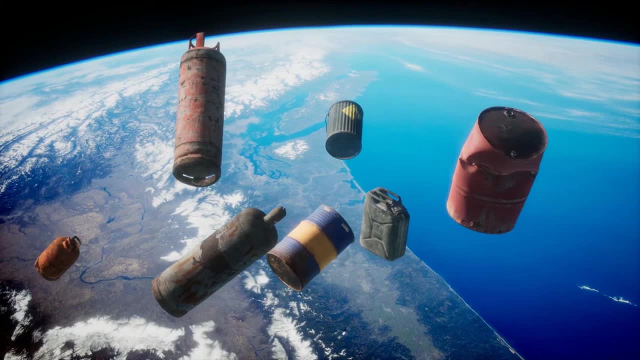 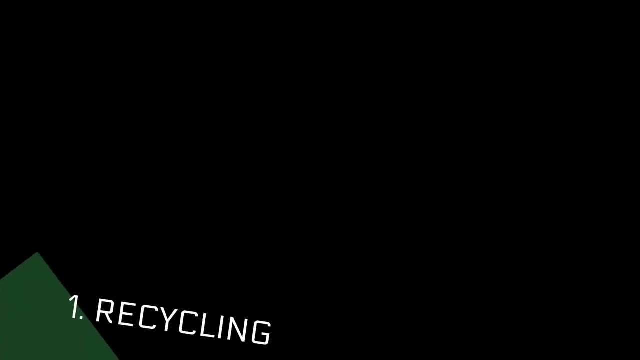 Waste materials created are a well-like trend. Proper. getting rid of wastes helps with maintaining your atmosphere free from pathogens that create illnesses and maintains it eco-friendly. Listed here are four techniques of appropriate waste management that may help you to keep your environment clean: 1. Recycling. 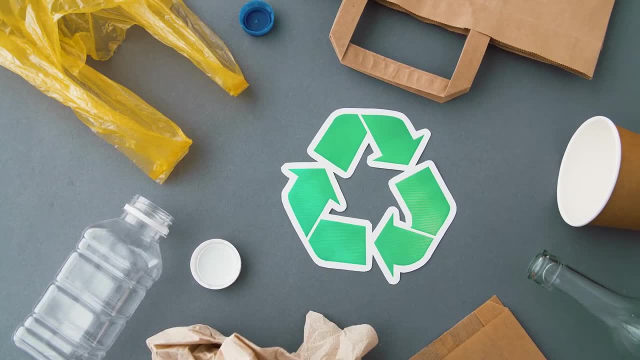 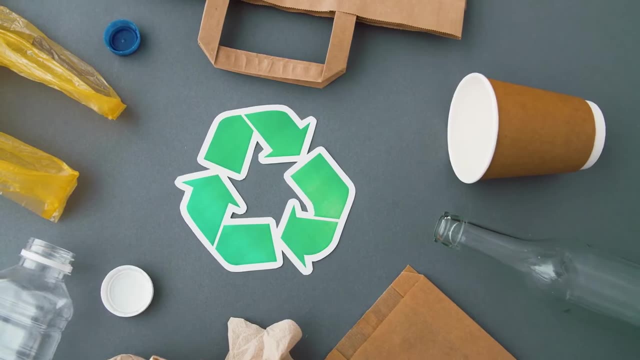 Probably the most anxiousness of waste management. recycling isn't pricey. also, it could be easily conducted on your part. When you perform recycling, you must be careful that your environment is clean and tidy When you conduct recycling. recycling you'll be able to avoid wasting sources, energy, and thus it will help reduce 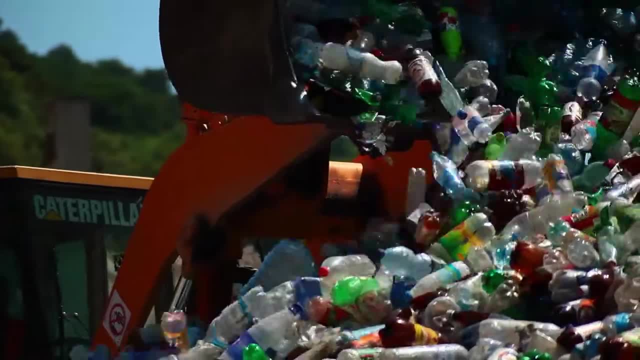 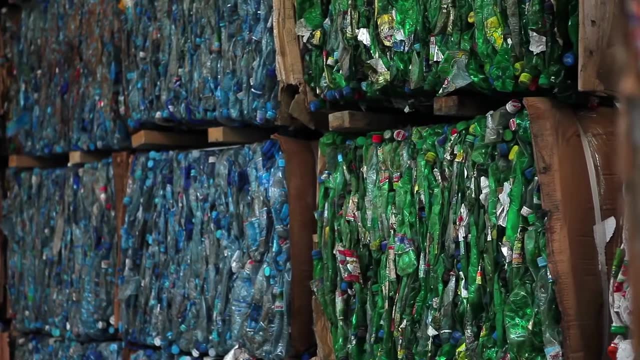 pollution. Also, you might cut costs whenever you recycle. Various materials that may be recycled include aluminum, plastics, glass and papers. If you want to lower the waste materials volume among the best ways you should do is to recycle, If you select recycling. 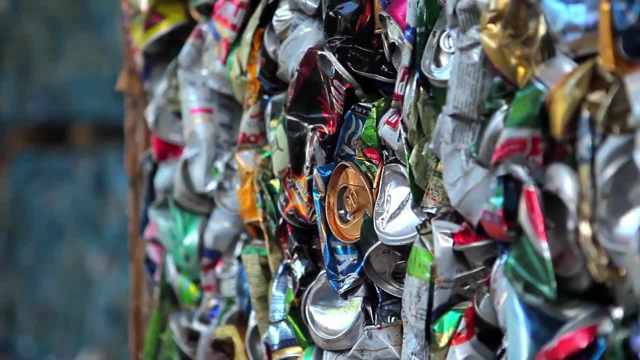 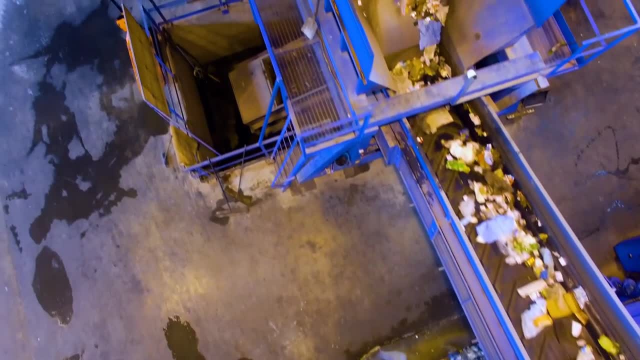 you can eliminate tires, asphalt and batteries in the waste materials. also, it stops them from being into the incinerator and landfills. The town of virtually every city motivates its citizens from taking up recycling. So be among these responsible citizens and reduce. 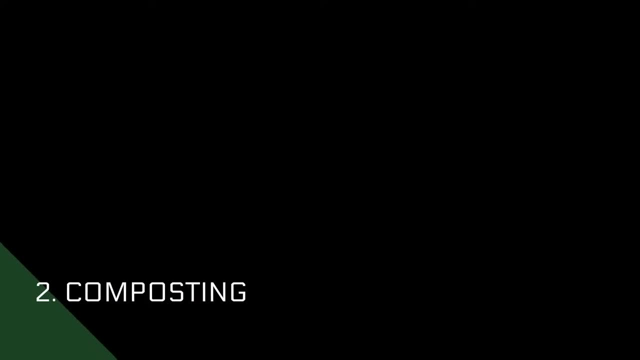 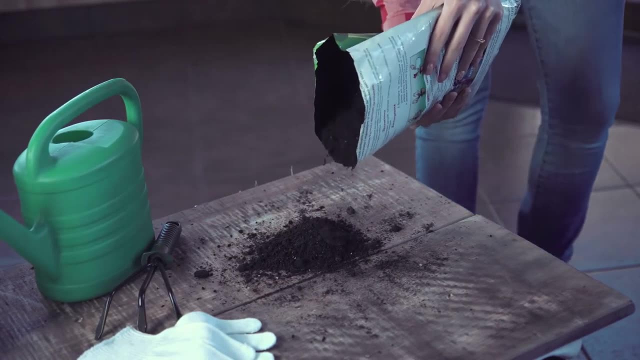 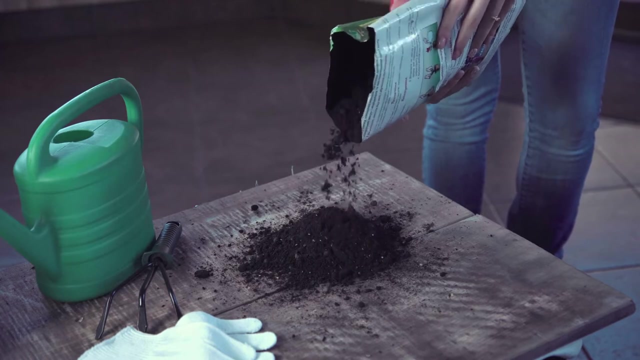 your waste through recycling. 2. Composting: Composting is the natural process that is devoid of any dangerous by-products. The procedure includes the break-lower procedure for materials into some organic compounds which may be utilized as manure. You might perform composting within your backyard. 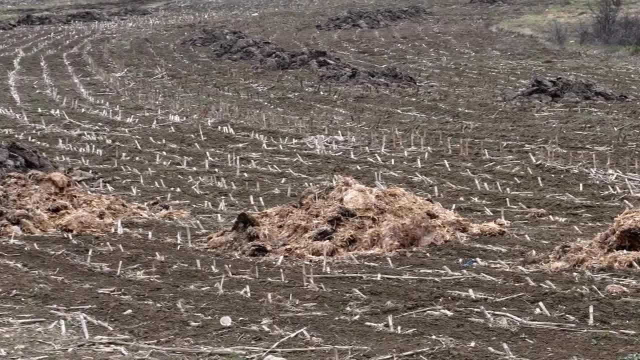 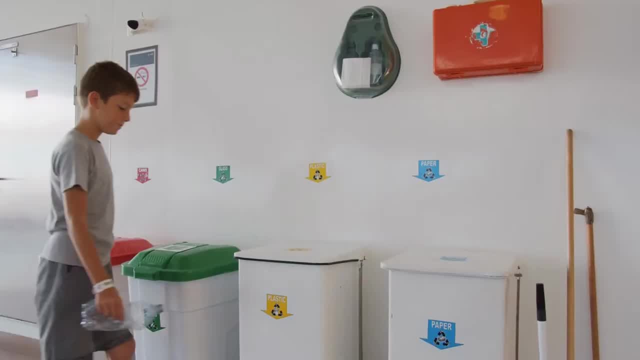 When composting, you can use grass, twigs, leaves and add vegetable and fruit skins and peels Soon after days. you need to realize that the types of materials have decomposed. You might employ this compost that's wealthy in nutrients so they can improve the soil. 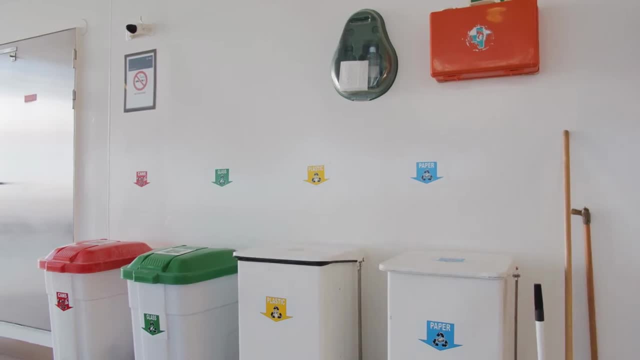 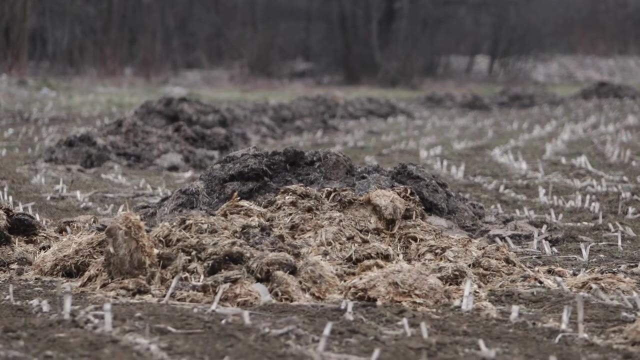 in your garden. What you're adding into your compost also has something to do with composting. The following steps help you start with composting and know what materials you should and must not include in the process. 1. Build a bin for the compost. 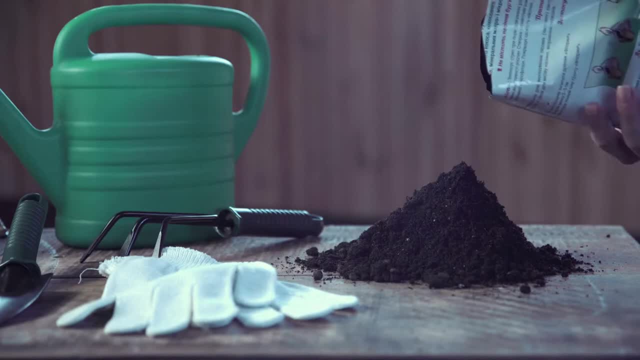 Though you can still successfully compost within a pile on the ground, using a container will keep the whole process neater and it helps in putting off animals. when you include food scraps in your composting process, Based on the bin's construction, it may also aid. 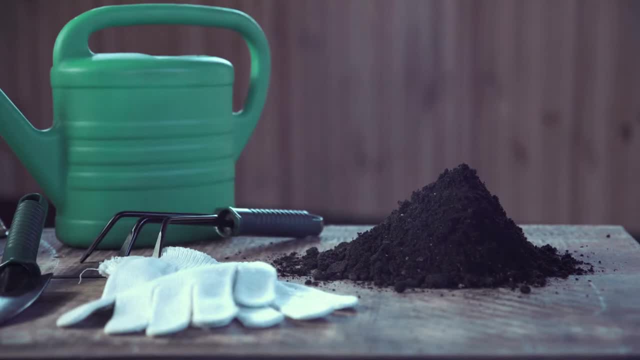 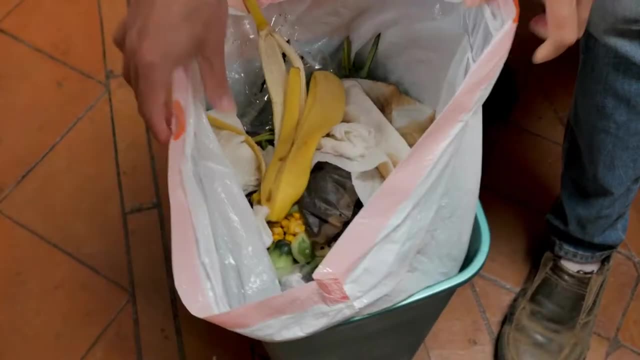 to regulate the temperature and moisture. Excellent. minimum pile size is at least one cubic meter or one cubic yard, but the pile may go more significant than this, while smaller-scale composting could be allowed to work. 2. Fill the bin with a balanced mixture for most excellent results. 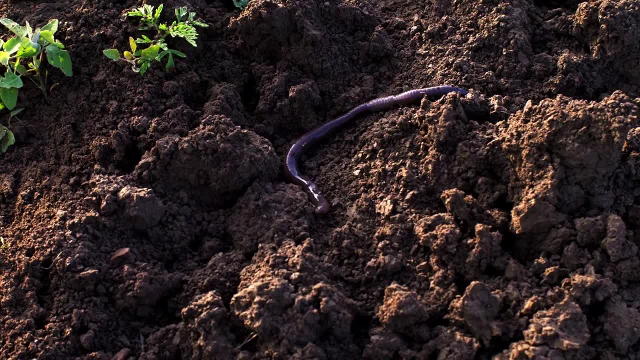 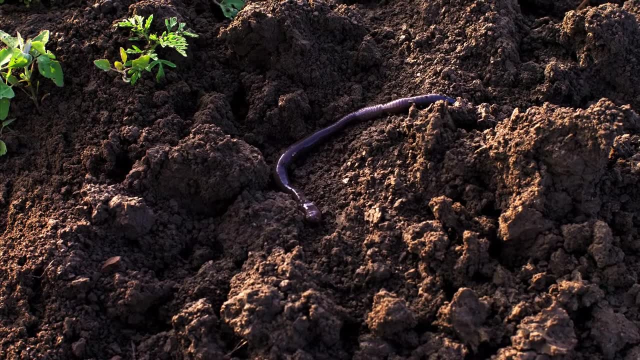 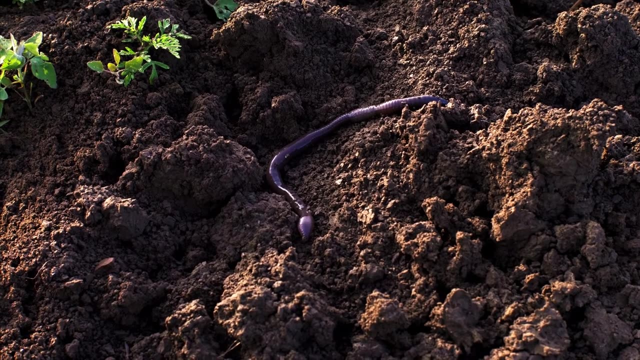 You may include the following into your mix: Green stuff for activating the heat process within your compost. Brown stuff to act as the fiber for the compost. Other items that could be composed that you might not have considered before, such as paper bags, paper towels, eggshells, cotton clothing, hair, human animals. Utilize all. 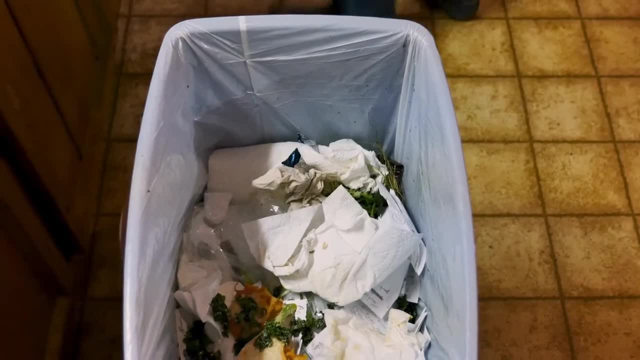 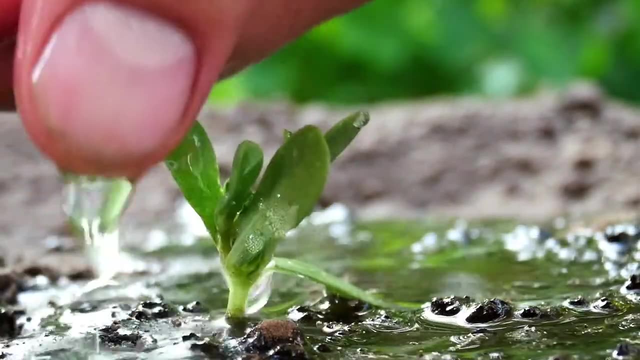 the items moderately Air. This helps deal with the smell produced by different bacteria. Anerobic compost for composting: This can attract phials that you do not want in your yard. Water: The pile must be around as damp as a sponge that has been squeezed out. 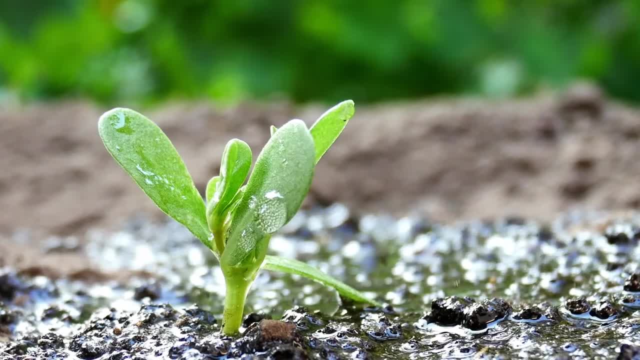 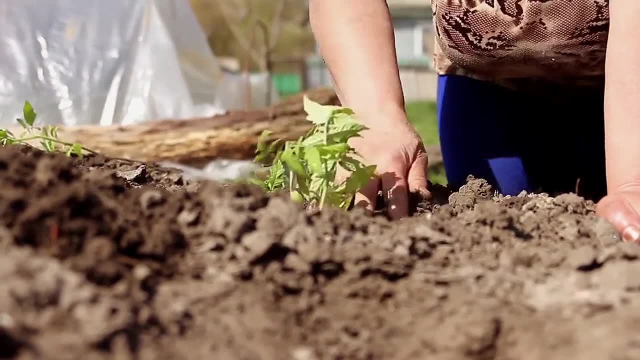 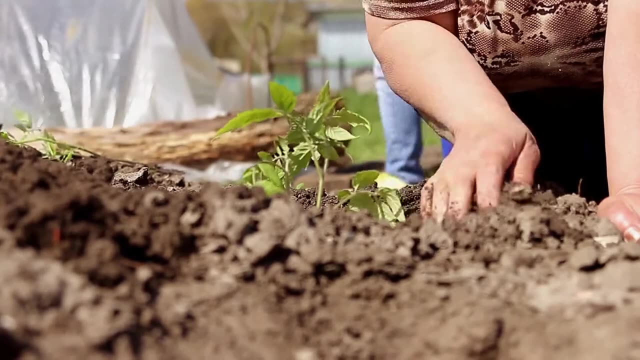 Temperature. The compost pile's temperature is extremely important and is a sign of the microbial activity of the process of decomposition. Starter or soil compost, It is not firmly necessary yet. recently completed compost between layers could aid to introduce the right bacteria to begin the composting process. 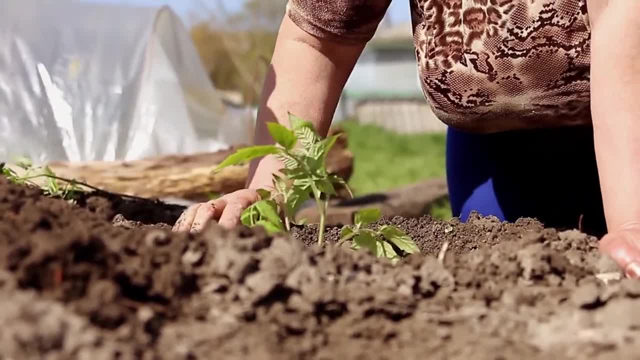 a bit more quickly When you are getting weeds. the soil that is left to decompose will be the first to decompose. The composting process will be done by hand, and the material that is left on the roots might be sufficient to serve. 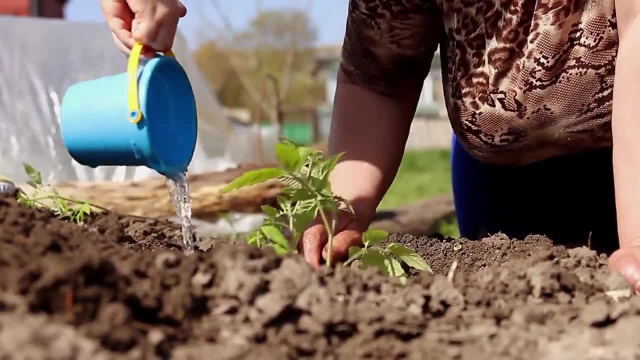 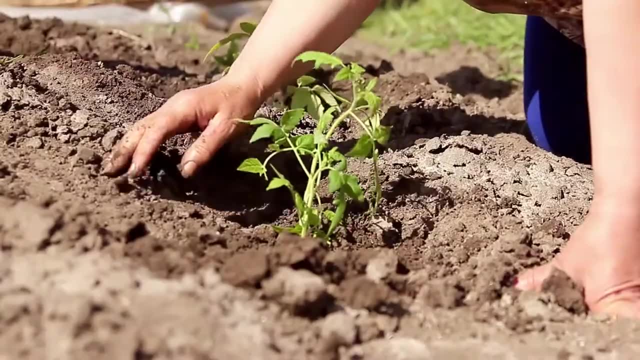 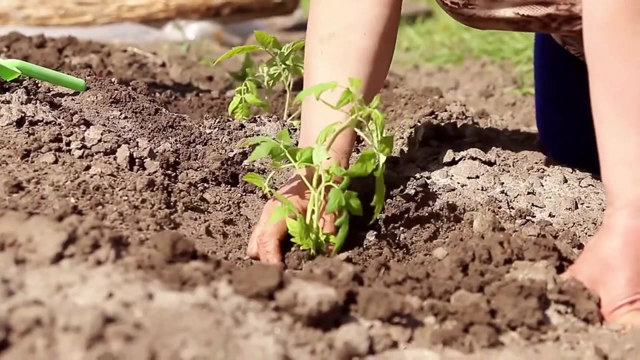 the purpose Mix of layer various materials within the container So that they could come in contact with each other. Also, with this you will be able to prevent any big clumps, Particularly avoid compacting together a large volume of green materials, as they may quickly become. 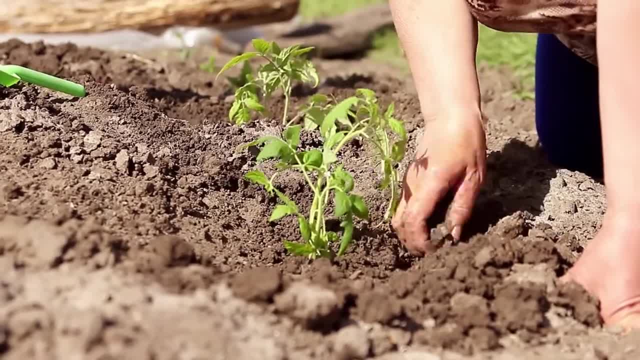 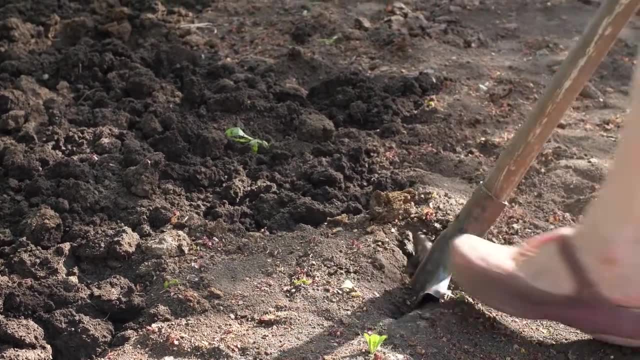 anaerobic. Turn the pile regularly, at least once each week or two. Decide whether you will add slow-rotting materials such as twigs, hedge clippings and sturdy branches, wood shavings, wood pruning and wood ash. 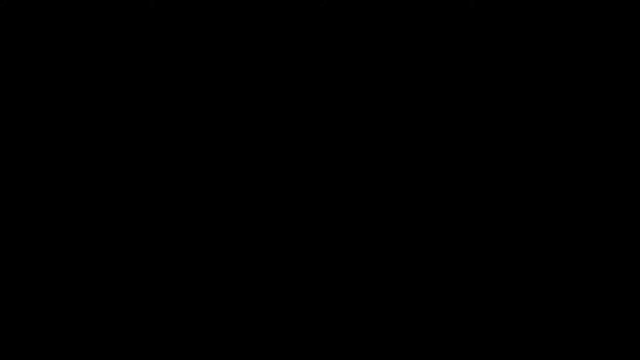 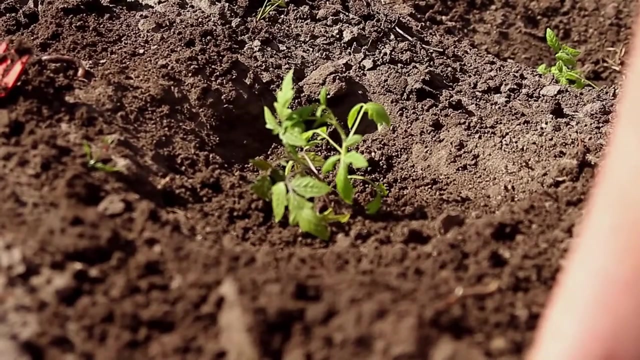 6. Know the things you should not compost. 7. Harvest the compost. When all goes well, you'll eventually find that you have got a layer of beautiful compost at the bin's bottom. Take this out and have it spread out on or dug into the garden beds.